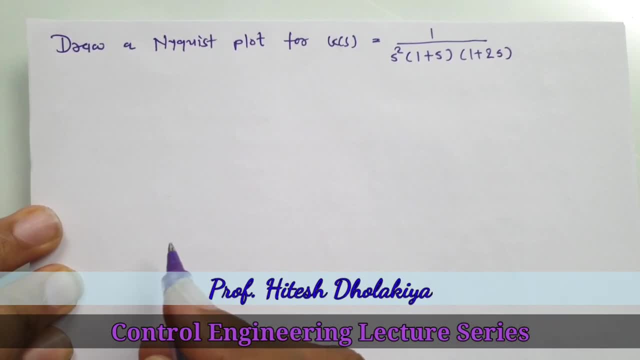 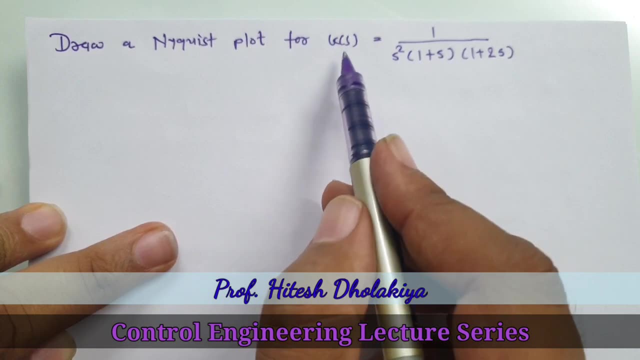 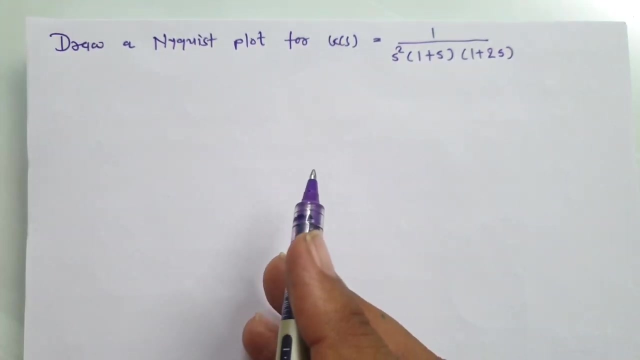 Welcome to control engineering playlist I. professor Ritesh Dholakia is going to explain you how to draw Nyquist plot in this video. So here we have been given with one system and we are delivered to plot Nyquist plot for this system. and I am giving you guarantee, after watching this video, you can plot Nyquist plot for any system, Right? So you just see this video from start to end. So Nyquist plot plotting is a. 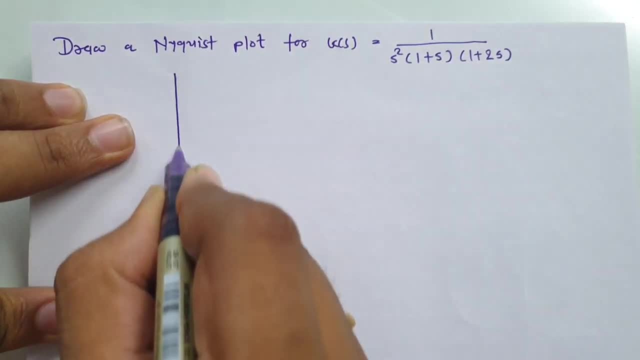 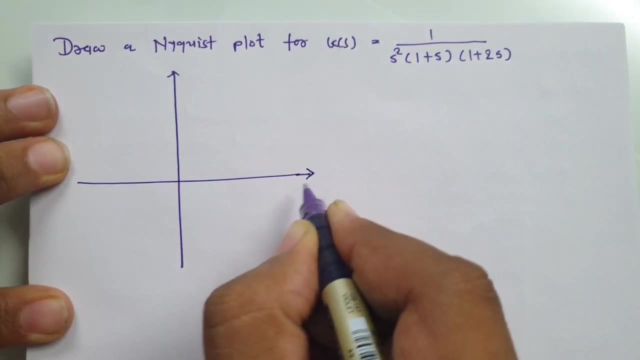 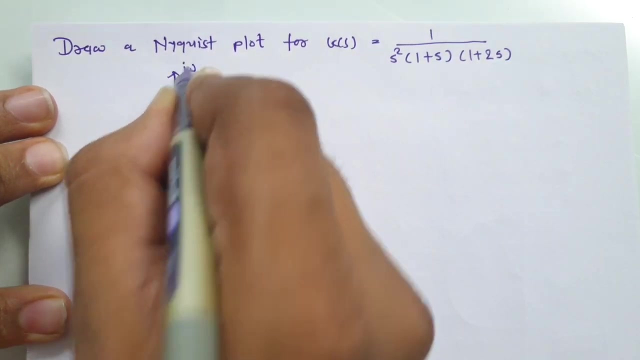 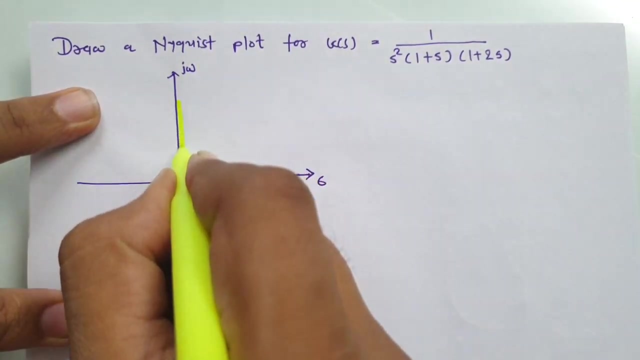 purely based on Nyquist contour. So let me explain you what is that Nyquist contour and how to follow all the steps one by one. So on real axis we have sigma and on imaginary axis we have j, omega, Right, And if you observe Nyquist contour, so that happens like this Right now. I am just making it by this. 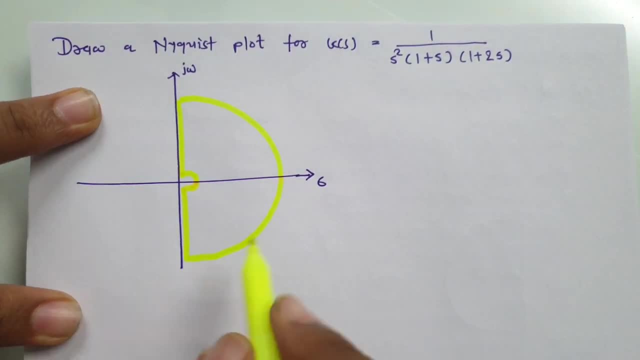 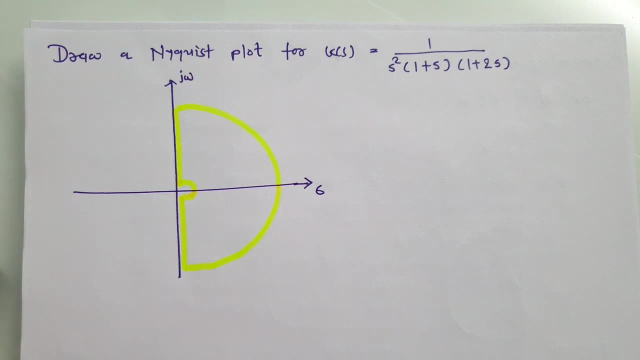 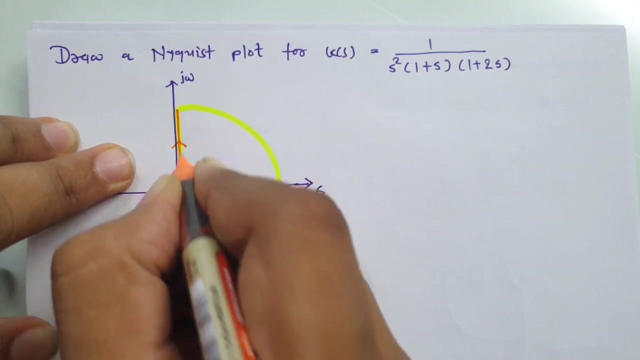 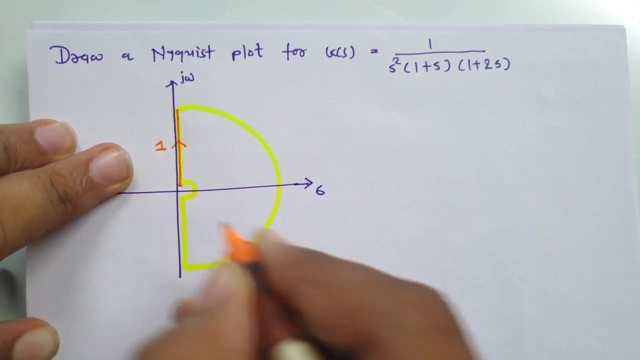 sketch pen. After that we will make it dark one by one, Right, Once we follow steps. So see, in this Nyquist contour, if you observe this portion Right. So in this portion we are delivered to place, s is equals to j omega. Let us say this is line number one, Right? So for this line number one we are delivered to place. 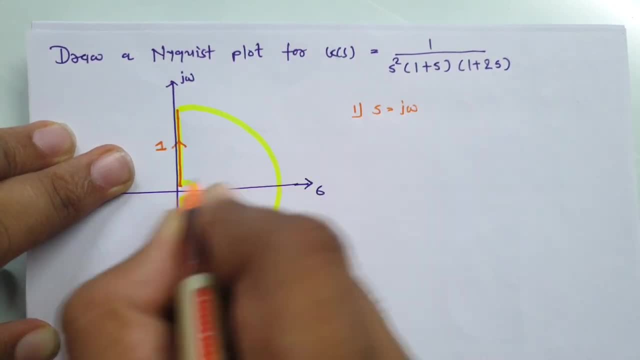 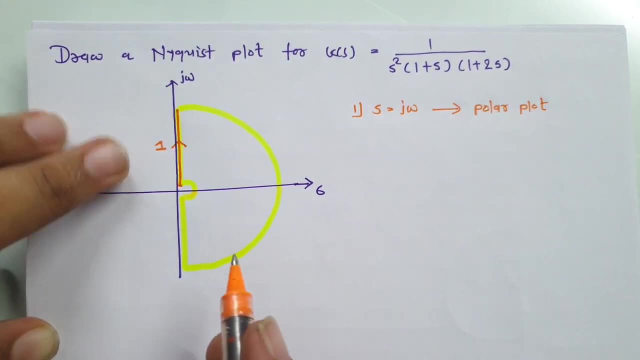 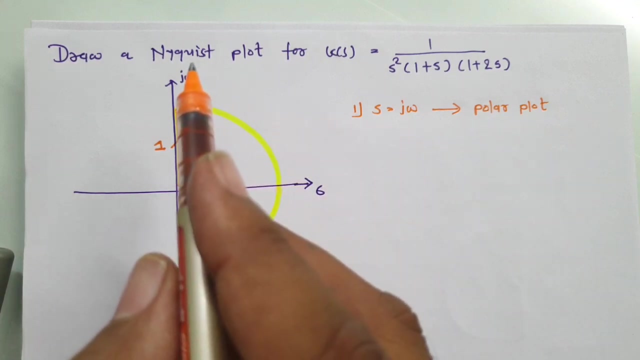 s is equals to j omega and s is equals to j omega means what it is: polar plot. i'll explain you how to plot polar plot. let me explain you the complete nyquist contour first, and then we will go for polar plot and then at the end i'll explain you how to plot nyquist plot. so this first line, that 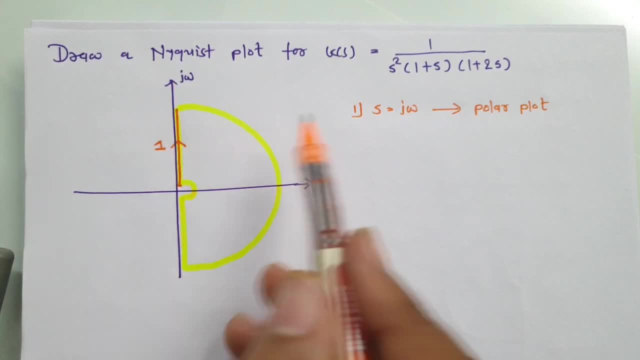 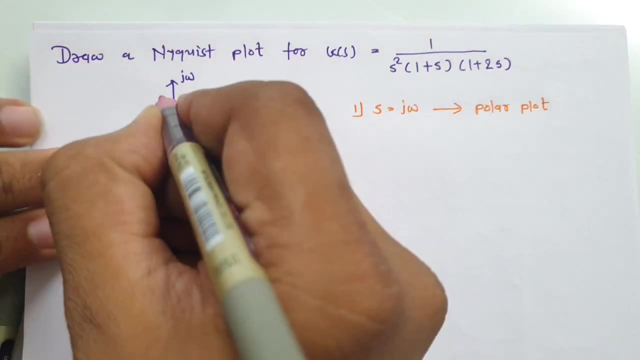 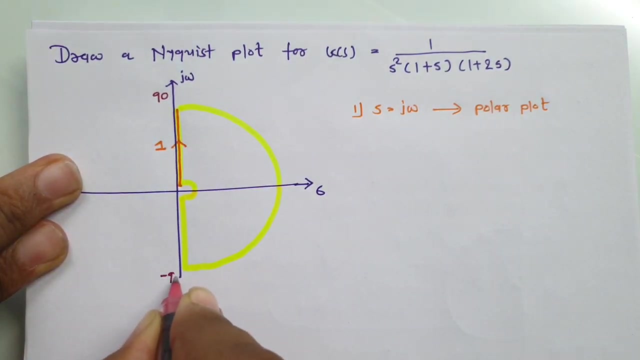 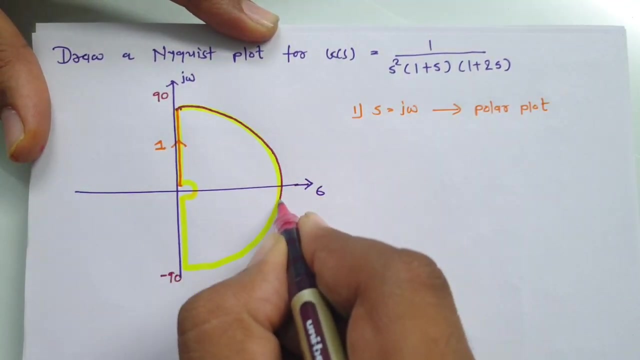 is there on j omega axis, right. so that is a polar plot section. now, here one should know: see, here angle is 90 degree and here angle is minus 90 degree, right. so in second section, see, this is infinite radius contour. is there right? and this infinite radius contour? 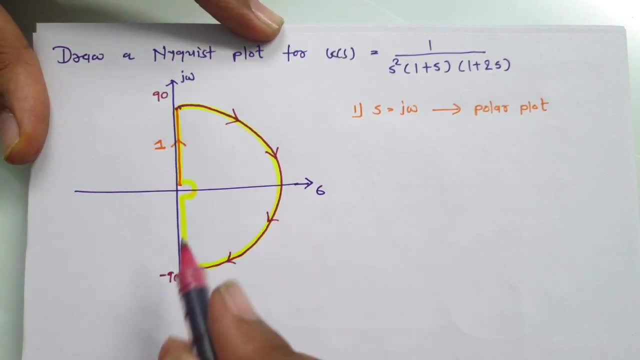 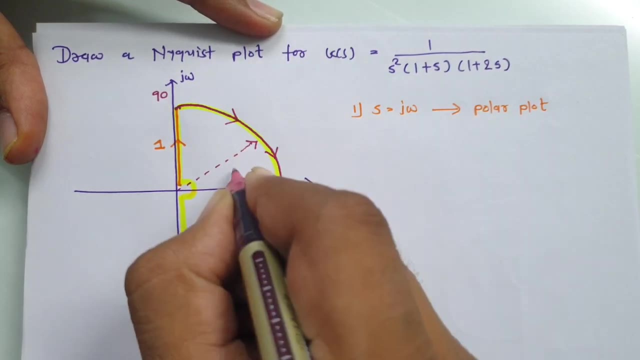 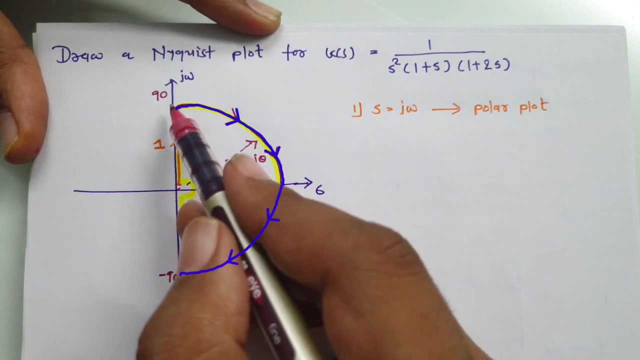 that happens from angle 90 to minus 90 and if you see the radius of it right, then that is infinite. so we can say this contour that is r into e, to the power j theta where r is going towards infinite and theta that varies from 90 to minus 90. you see, that is how it is happening, right? so in second, 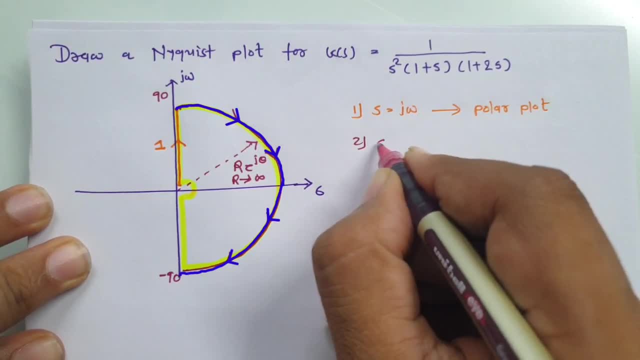 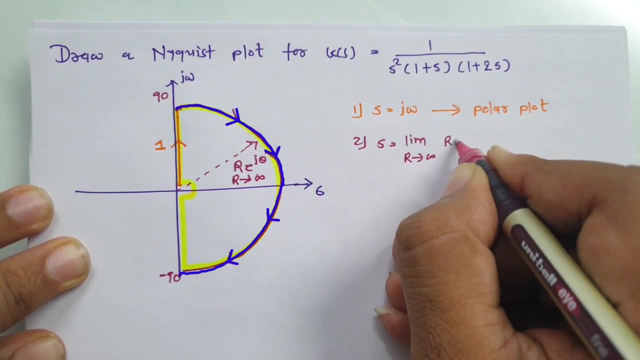 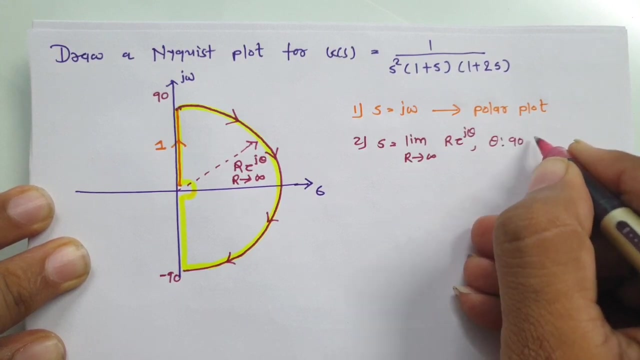 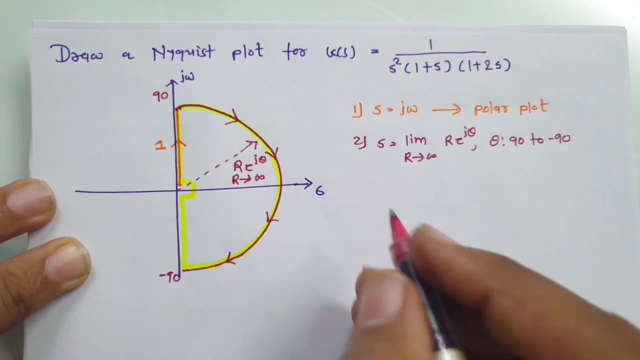 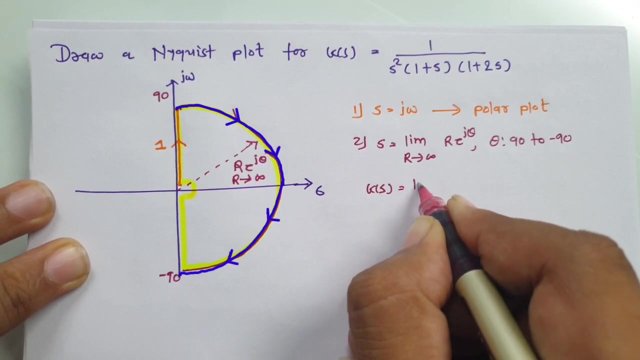 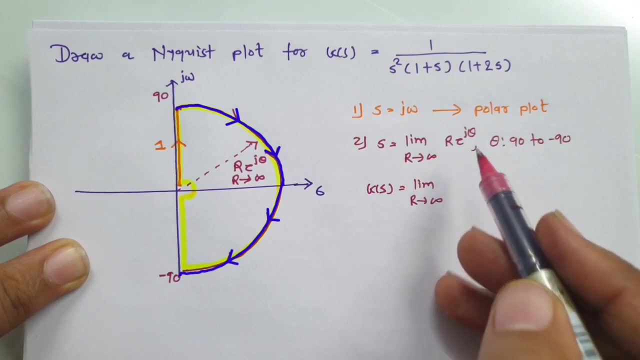 step, we will be placing s, that is limit, radius tends to infinite, r e to the power j theta, where theta varies from 90 to minus 90, right and now we will identify this system right. so you see, this system g of s right over here, that will be limit r tends to infinite. and now, instead of s, we will be placing r? e to the. 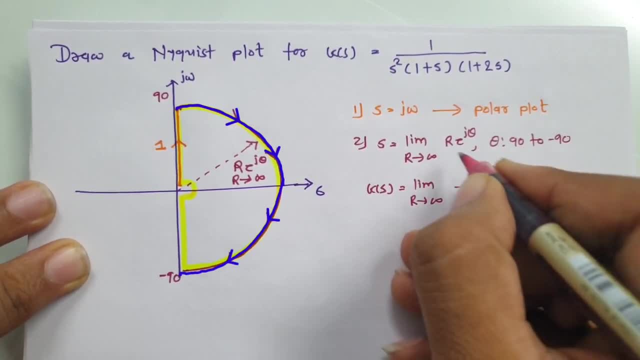 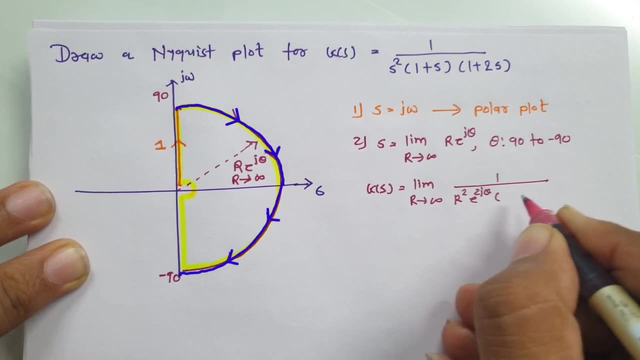 power j theta, so 1. divided by now you see s square. that will be r square into e to the power 2 j theta into counts. 1 plus s is r into e to the power j theta into 1 plus 2 j 2 s, so 1. 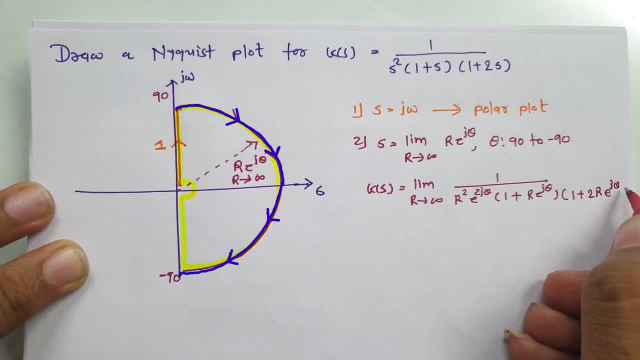 plus 2 into r, into e to the power j theta, right. so this is what system which we have for second line. now we need to simplify this. so r is tending to infinite. so to simplify this, all we'll be doing is we'll be taking r? e to the power j theta common from this term and 2 r e to the power j theta. 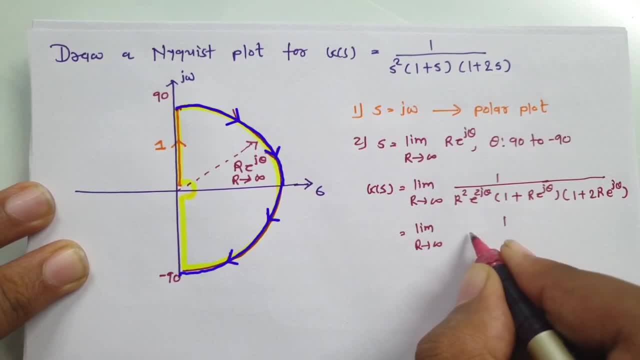 from this term right. so now you see little simplification version of this. that will be: 2 r is to 4 e to the power 4 j theta into 1 plus 1 by r e to the power j theta and 1 plus 1 by 2 r e to the power j theta. right as I have to. 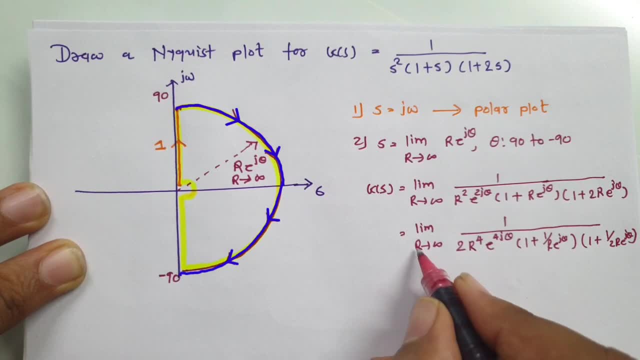 common from this two term. now, if you place r tending to infinite, so this will be 1 plus 0 and this will be 1 plus 0. so I can say now this term, that is r, tends to infinite, 1 by 2, r to the. 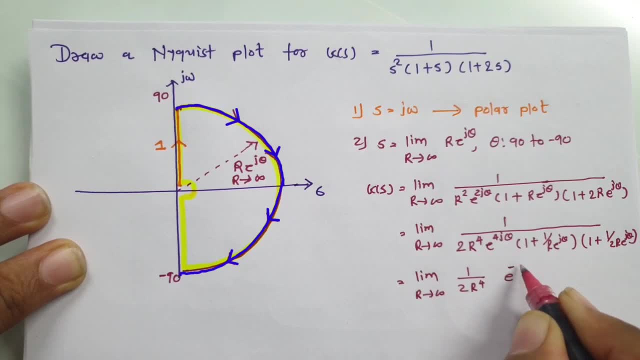 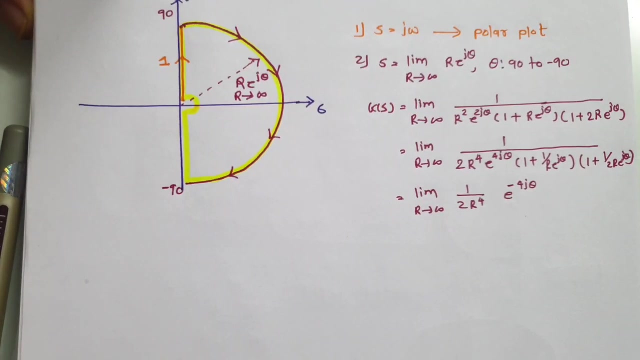 power 4. and you see, here I am writing e to the power minus 4 j theta. in numerator it will be minus 4 j theta over here right now we need to understand what is the meaning of this terms. right, so you just see what is the meaning of this terms. see, this explains you magnitude. 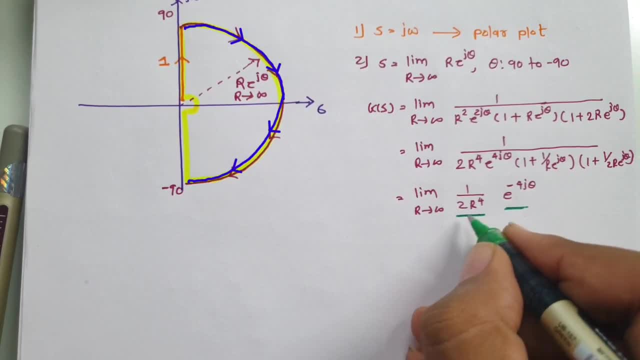 and this explains you phase. so you see, if r tending to infinite, 1 by infinite raise to 4, so that will be 0, so magnitude over here that is 0, right. and if you see this term, so that is having e to the power, 4, j, theta, and here you see, theta varies from: 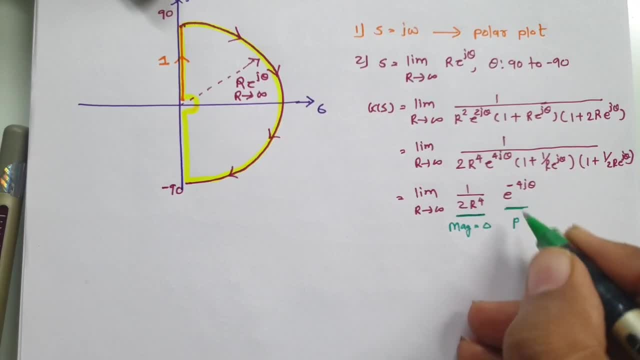 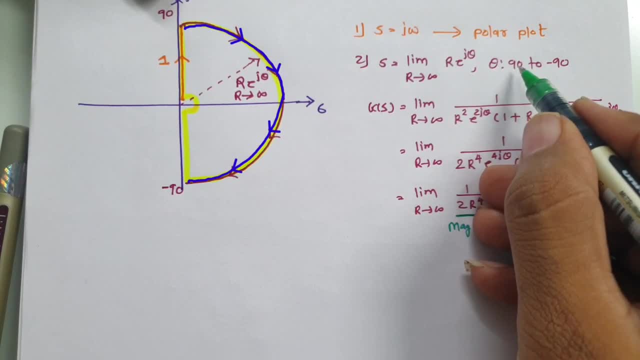 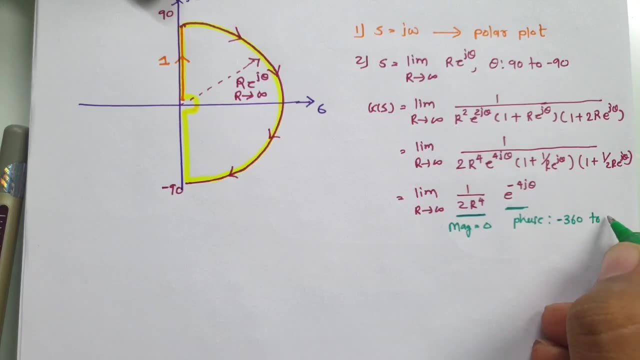 so 90 into minus 4, so that is minus 360. to minus 90 into minus 4, so that is 360. so now phase will vary from minus 360 to plus 360, and when you plot nyquist plot in that if phase is varying from minus angle to plus angle, then you will have to. 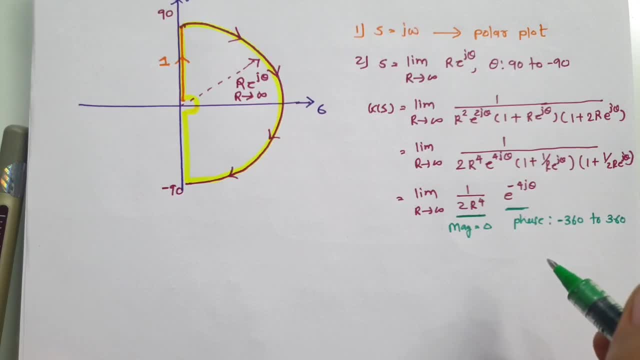 have anti-clockwise circle, right, but here you observe minus 360 to plus 360 variation is happening means two circle will happen, right, and that will happen in anti-clockwise direction, as minus 360 to plus 360 is happening, and that will happen in anti-clockwise direction. 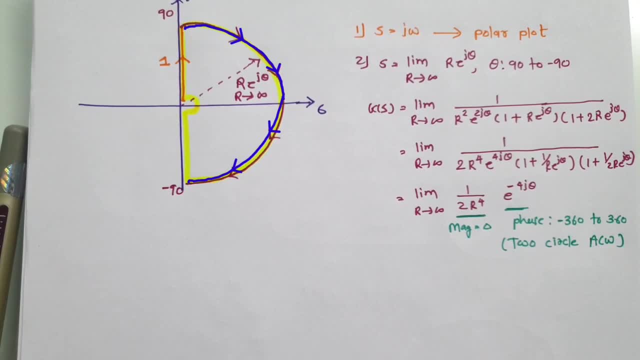 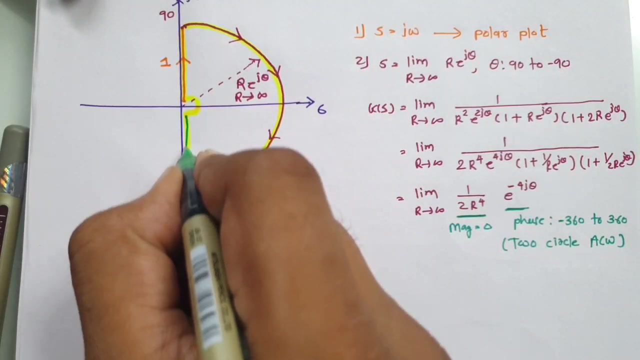 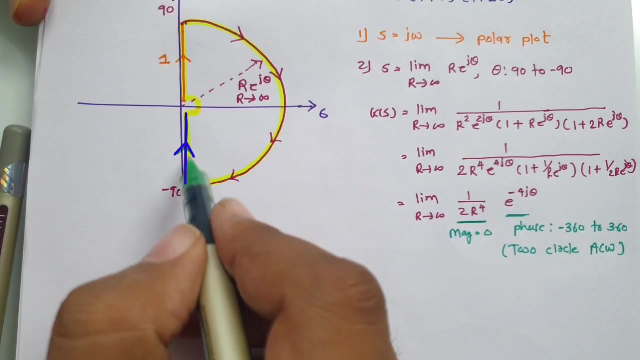 minus 360 to plus 360 angle variation is happening. so i'll explain you how to have that in nyquist plot diagram. now you see third portion. so that is this, and in this you see now our uh nyquist contour that is having s is equals to minus j omega right. this is j omega x and this is. 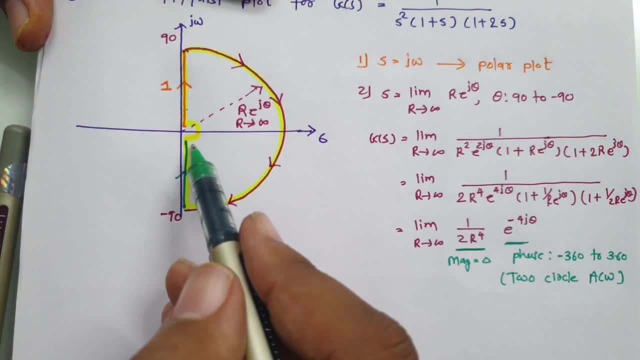 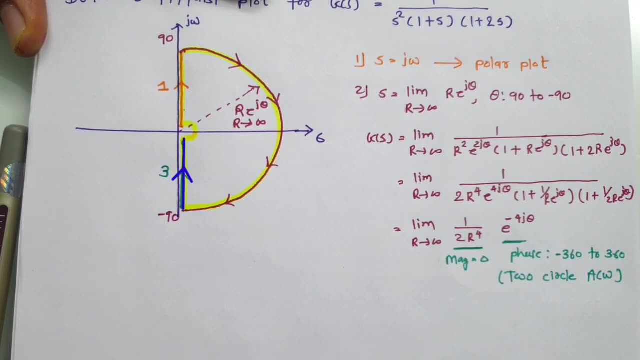 this is positive j omega axis and this is my minus j omega axis. so when you plot this third line, right? so in this third line you will have to have s, is equals to minus j omega and this is inverse polar plot. so once you have polar plot, we can have inverse polar plot. so i'll explain you. 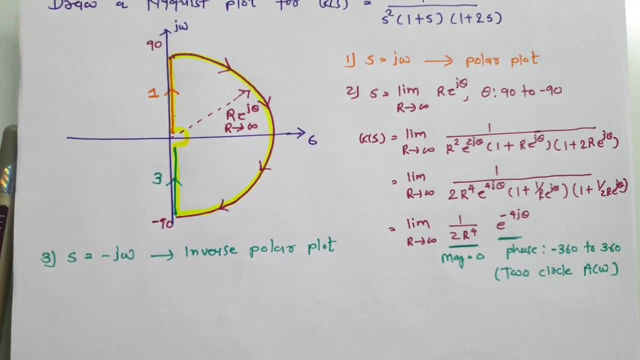 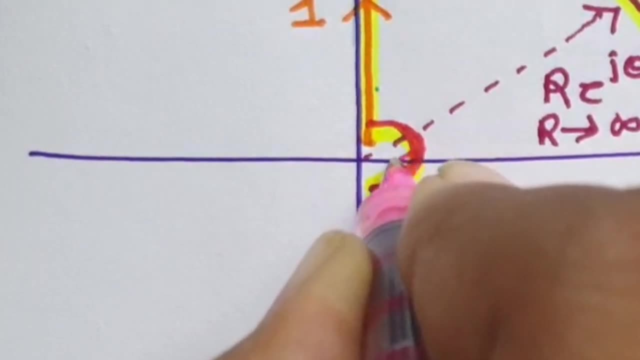 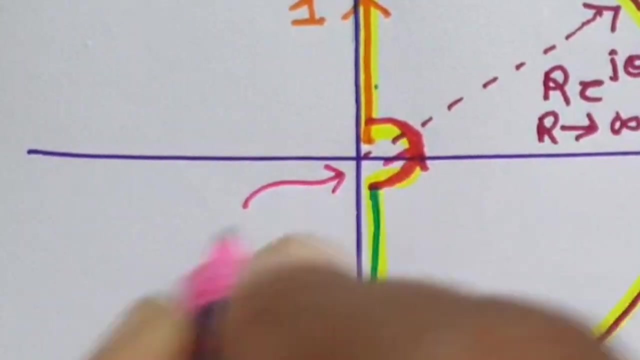 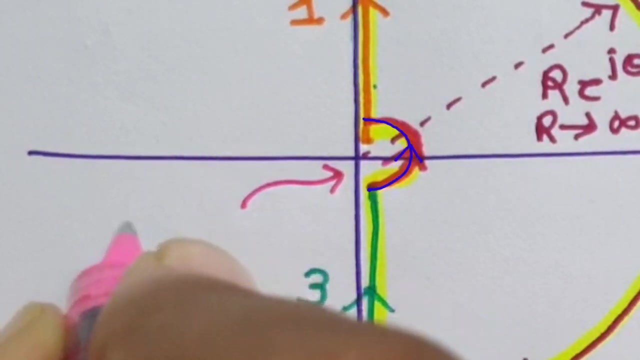 how to have that inverse polar plot and this fourth part, that is, this small circle, you see, and this small circle that is happening from minus 90 to plus 90, right, and if i write about this small circle, then that is having radius which is tending towards 0, so i can say it is having radius r. an angle varies from j theta. 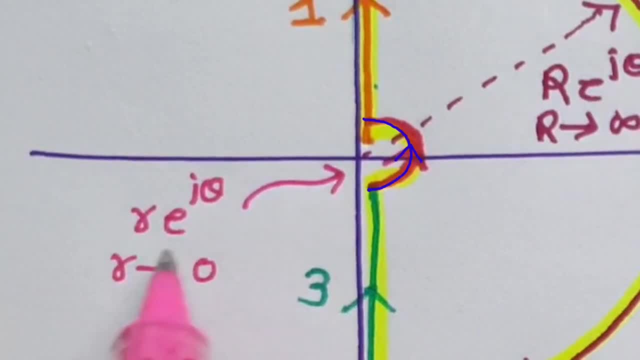 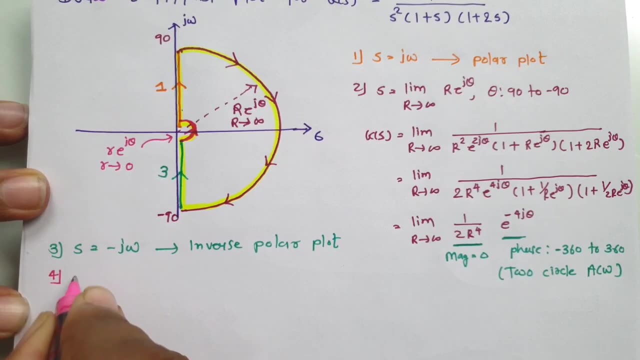 where small r tends to 0 and angle will vary from minus 90 to plus 90. so let me write that fourth term, where here we'll be placing s, is equals to limit r tendings to 0. small r e to the power j theta, where theta will vary. 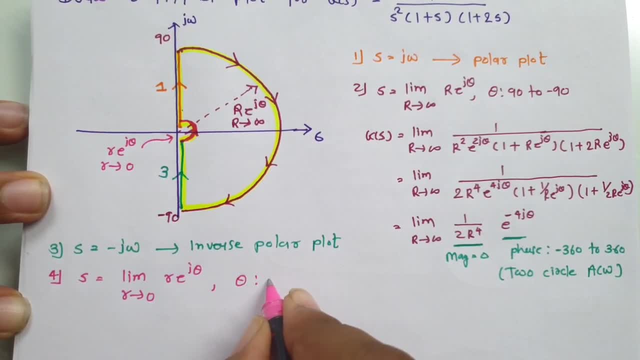 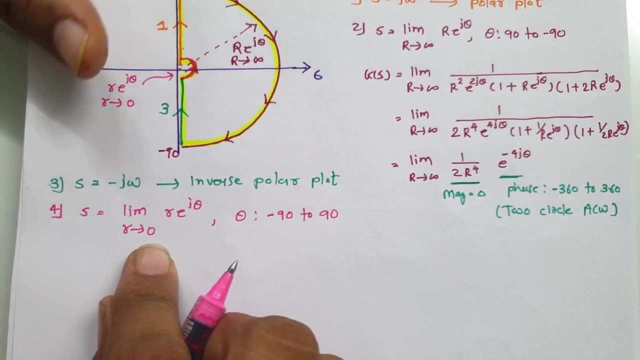 from minus 90 to plus 90 and by placing this in transfer function we can have this angle which is tending towards 0, and angle will vary from minus 90 to plus 90. so we have a value of magnitude and phase variation. so let us have that g of s in that. 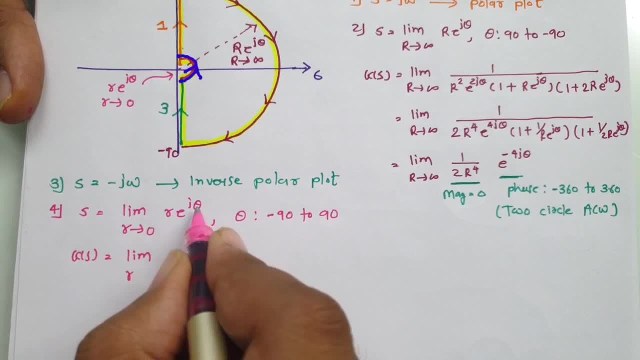 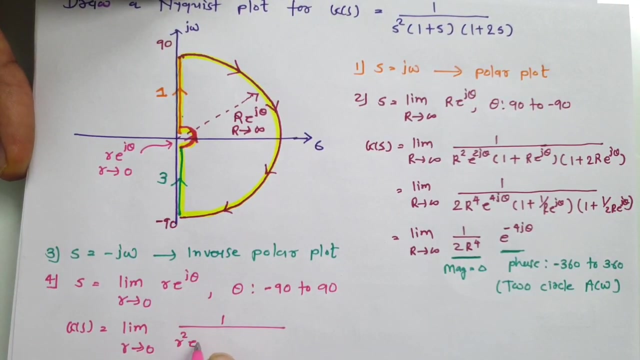 we'll be placing. s is equals to r e to the power j theta, so r tending to 0 and in transfer function. you see i'm placing it, so s square is there, right. you see, here s square is there, so here it will be r square e to the power 2 j theta into 1 plus. 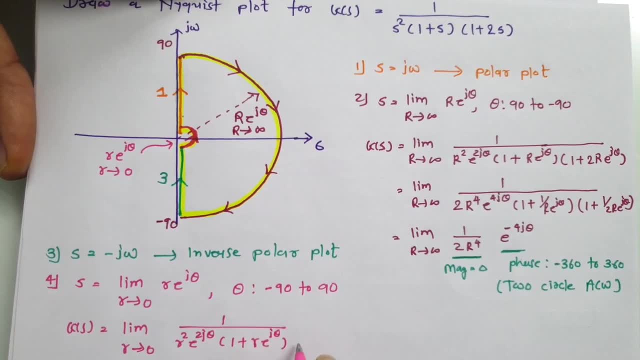 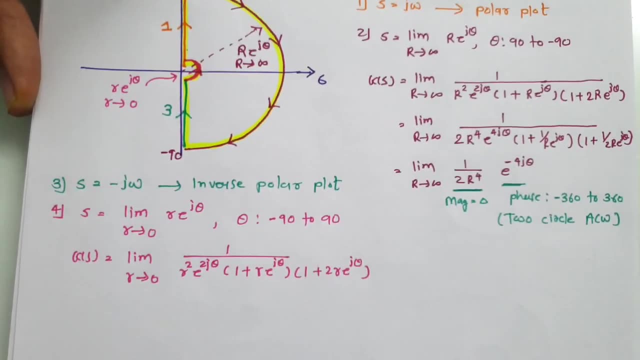 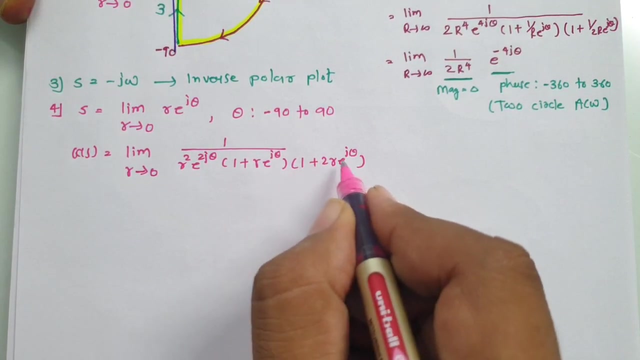 r e to the power j theta into 1 plus 2 small r e to the power j theta. now let us simply verify this so you see, if you place r tending to 0, so this term will be 1 plus 0 and this term will be 1 plus 0, so we have limit r tending to 0. 1 by r square into e to. 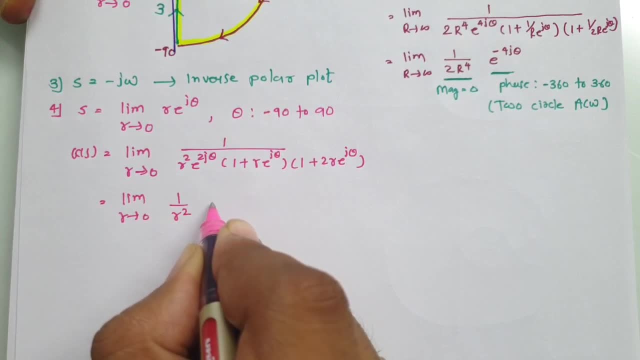 the power. now you see e to the power, 2 j theta. that is there in denominator. so we have limit r, tree, small r. e to the power, five t letters. now you have same formula here, so denominator. So here I should be writing minus 2 j theta over here. Now in this again you: 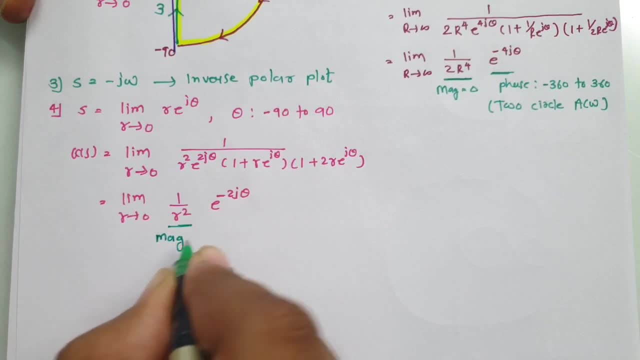 see, this is representing magnitude and this is representing phase. Now you see magnitude 1 by 0, so that is going towards infinite, and here you see phase variation. So theta varies from minus 90 to plus 90, and here angle is minus 2 theta. So if you multiply minus 2, 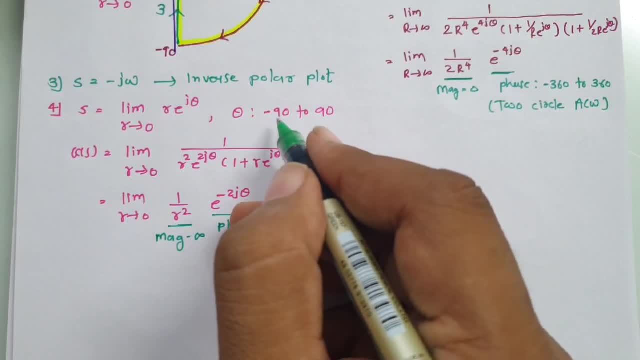 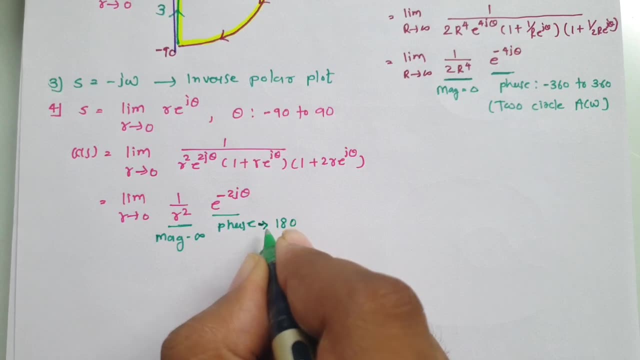 theta. So now phase will vary from minus 90 into minus 2, so that will be plus 180.. Phase will vary from plus 180 to 90 into minus. 2 means minus 180.. So phase will vary from plus 180 to minus 180.. 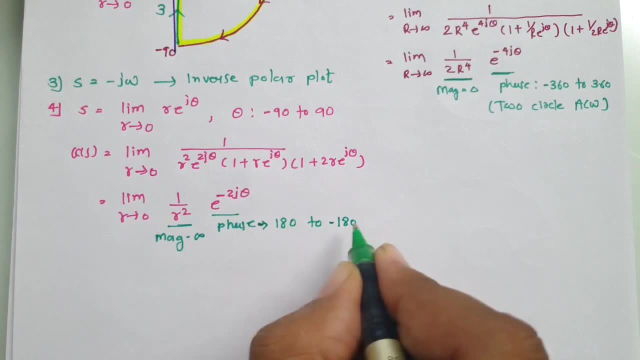 And as phase is varying from positive angle to negative angle, there will be clockwise direction circle And angle is varying by 360 degree, means one circle will happen, Right. so here one circle will happen in clockwise direction, So positive to negative variation. 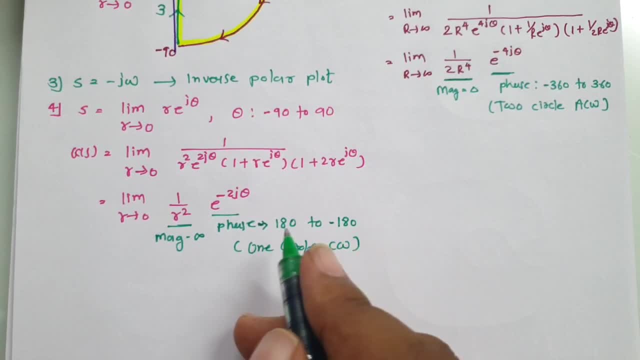 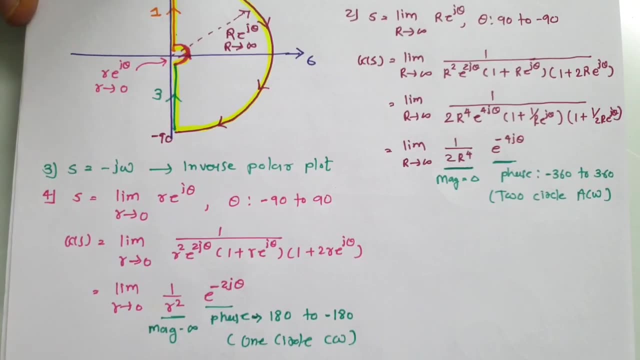 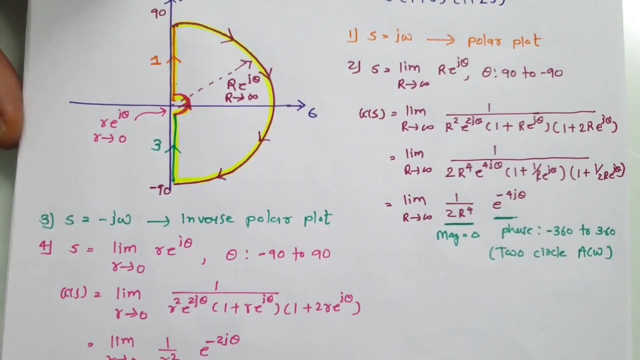 means clockwise direction, and 180 to minus 180 means total 360 rotation means one circle will happen. so now this four steps, that is clear. and now, once you have this first step, which is a plotting of polar plot, we can completely plot Nyquist plot over here, right? 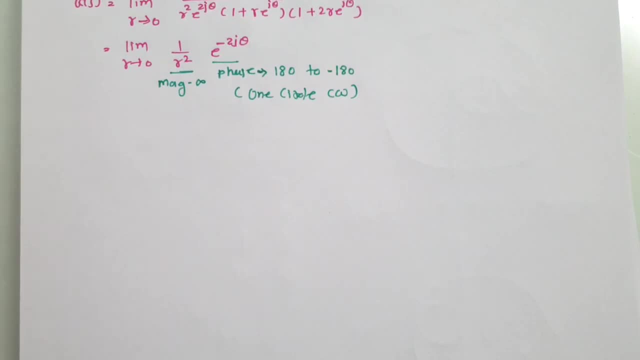 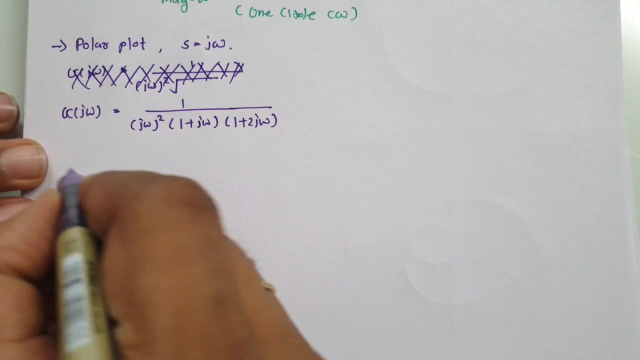 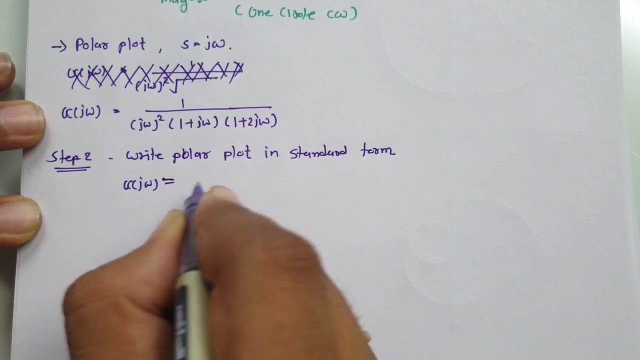 So let us have a polar plot of this. that is to write: s is equals to j omega, right? So now we have g of j omega. let me write that Now, in next step, we will be writing polar plot in standard form, right? So standard form, that is g of j omega. that is equals to magnitude of this into phase. 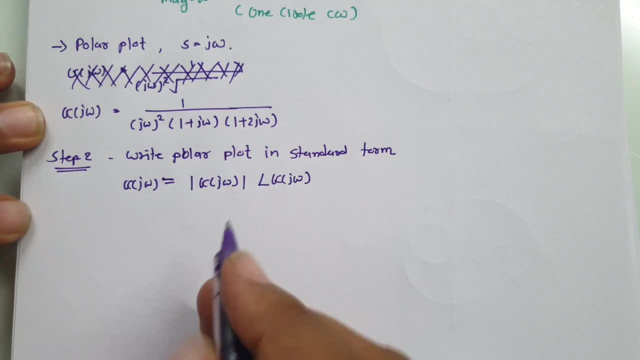 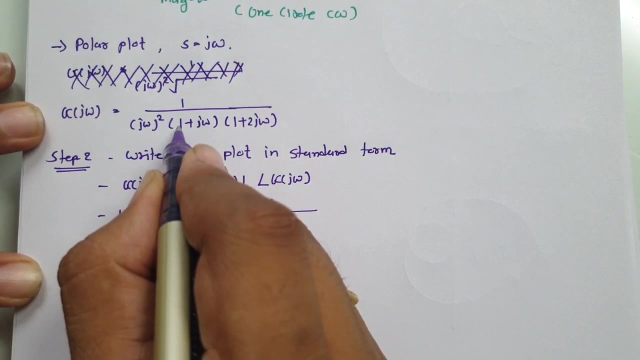 of g of j omega right Now, what will be magnitude? So magnitude g of j omega, That will be 1 divided by. you see now j omega whole square, so that will be making it to omega square. and now you see 1 plus j omega. so magnitude of that: that will be square root. 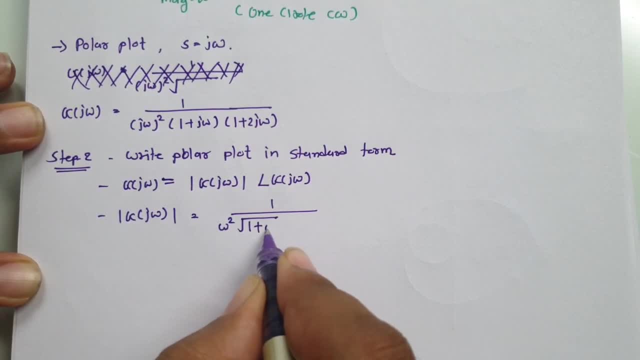 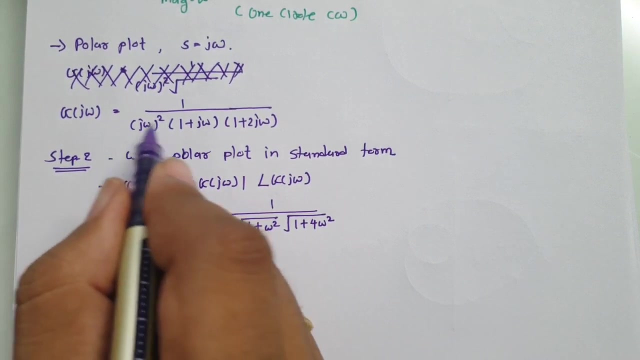 of real part square plus imaginary part square, so 1 plus omega square into magnitude of this, that will be 1 plus 4 omega square and phase, that is angle of j omega. So now you see, So that will be 1 divided by j omega square. so there are two poles at origin, so pole is: 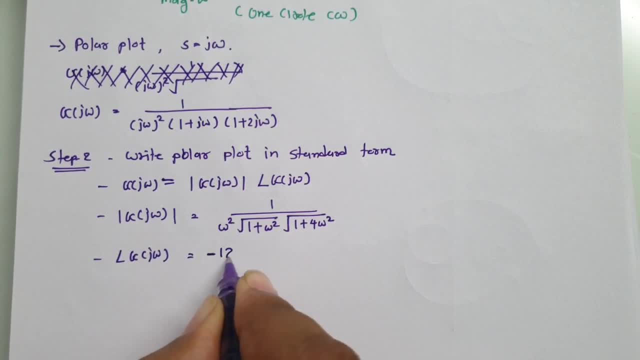 having negative angle. so for two poles it will be minus 180 and for 1 plus j omega pole that angle will be minus 10 inverse omega and for this second pole this will be minus 10 inverse. So omega square plus 2 omega. and how it is happening? 10 inverse. imaginary component divided. 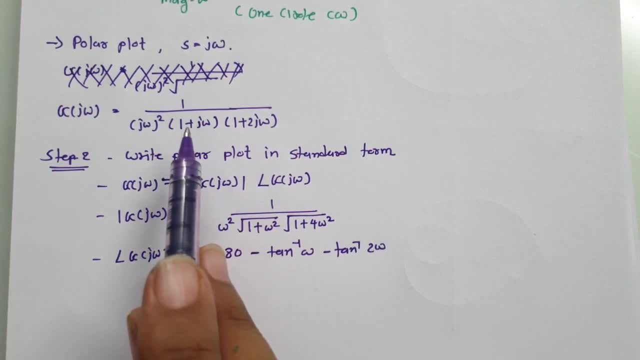 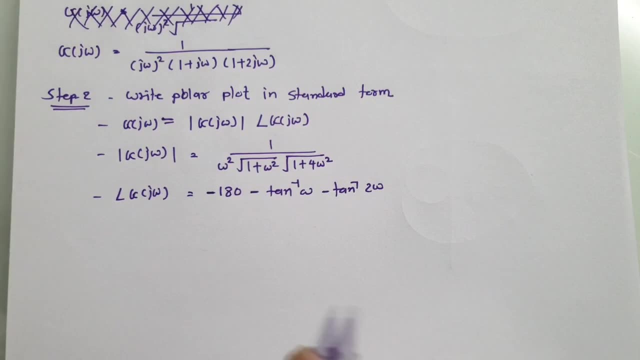 by real component. Real component is 1 and imaginary component. that is what you can see over here and as per that, I have written this phase. Now, once we have this magnitude and phase, all we can do is we can identify two important points. So we are delivered. to find omega is equals to zero point. 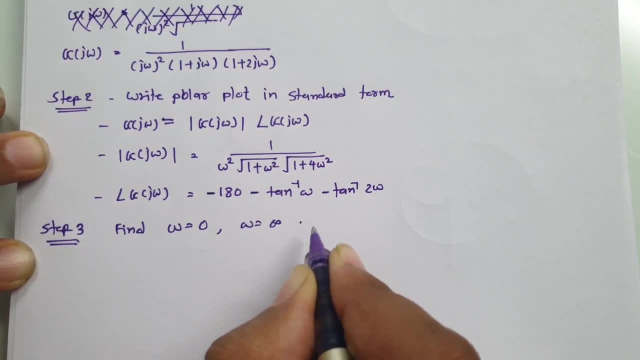 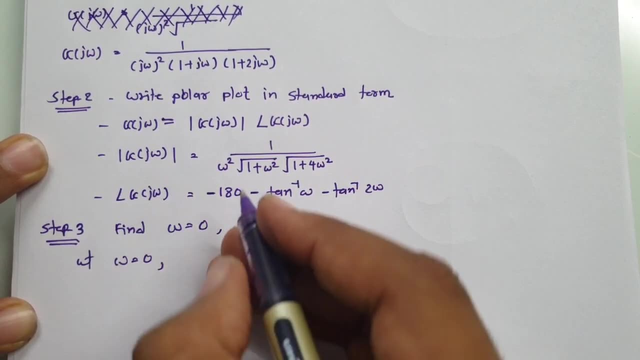 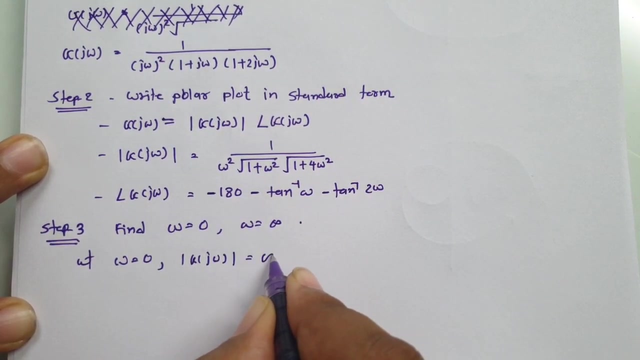 And we are going to write that: And omega is equals to infinite point, right. So at, omega is equals to zero. if you place zero, what will be magnitude? magnitude will be 1 by 0, so that will be infinite. And what will be phase? you see, if you place 0, so 10 inverse 0, that is 0, right? 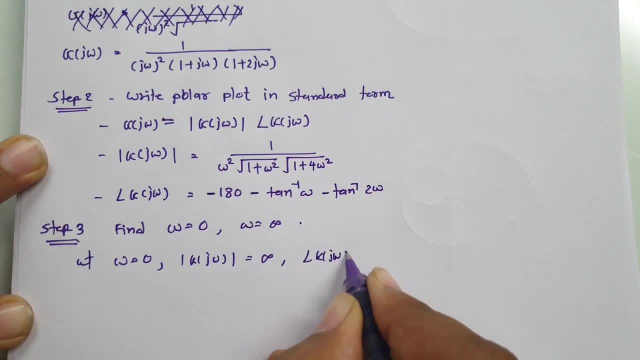 So this will be having phase That is minus 180. And if you place omega is equals to infinite in this, So 1 by infinite, so that will be making magnitude 0. And if you want to identify phase g of j omega, then you see minus 180 and 10 inverse infinite. 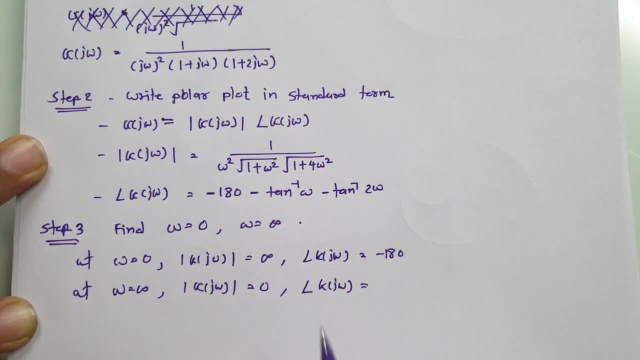 So this will be minus 90 and this will be again minus 90.. So that will be minus 360.. Okay, So now we have two essential points Now to identify intersection to real and imaginary axis. first we need to separate real part and 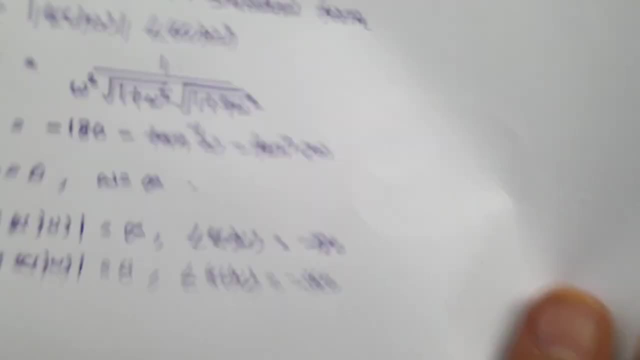 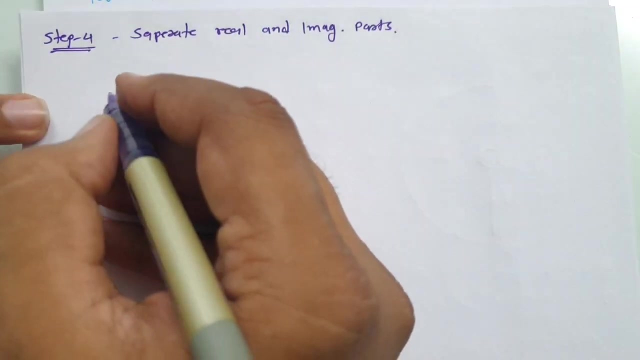 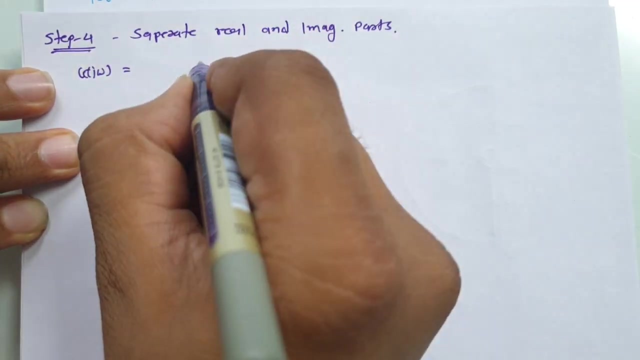 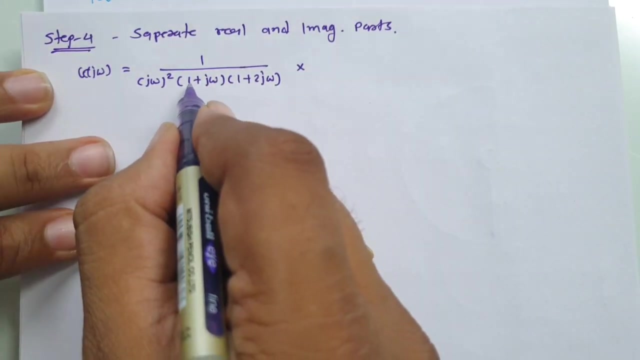 imaginary part, right. So let me explain you that. how to separate that, step by step. So to separate real and imaginary part, all we need to do is we need to multiply complex conjugate of denominator, Right. So here my function is. so to separate real and imaginary part, I need to multiply complex. 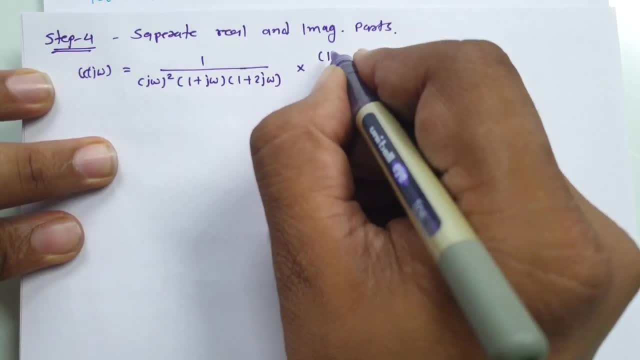 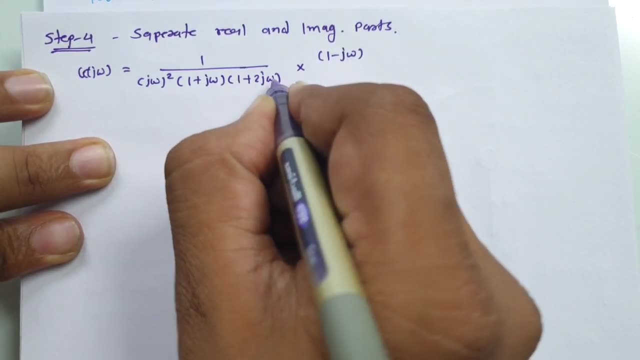 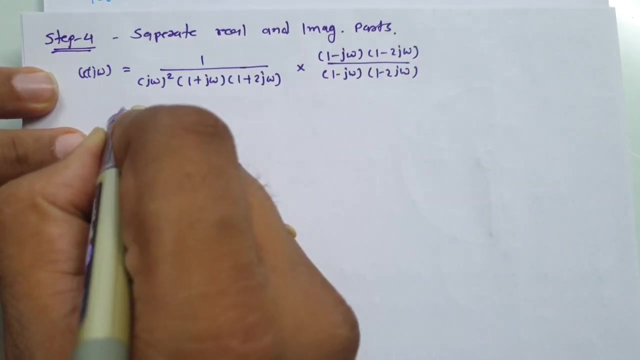 conjugate of denominator and divide it. So now you see: 1 plus j omega. so I'm multiplying and dividing 1 minus j omega and 1 plus 2 j omega. so I'm multiplying and dividing 1 minus 2 j omega. So now what will happen? you see? 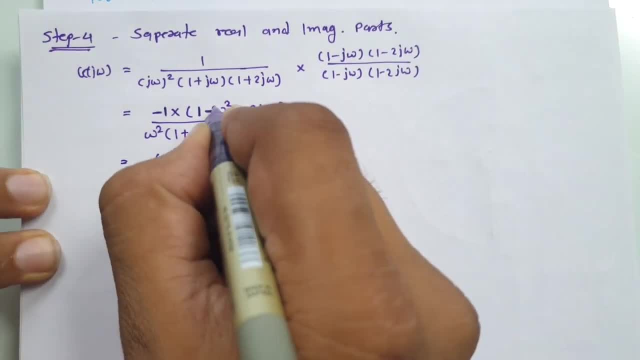 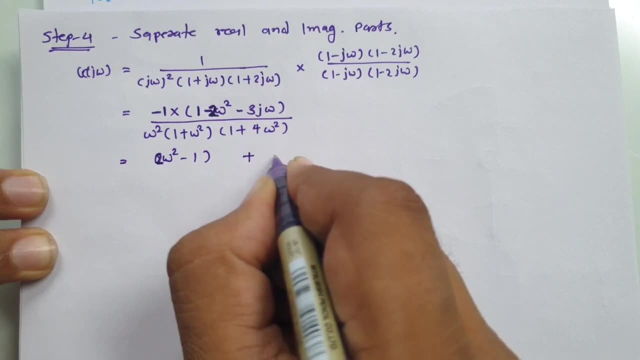 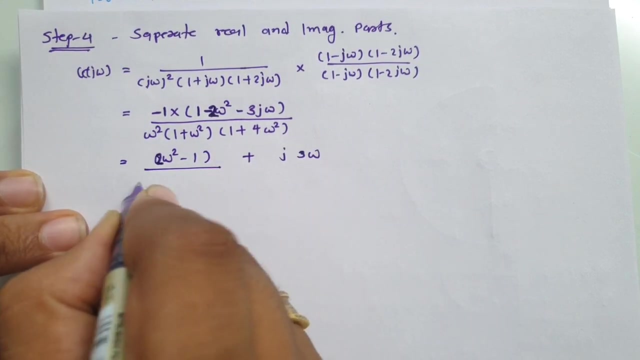 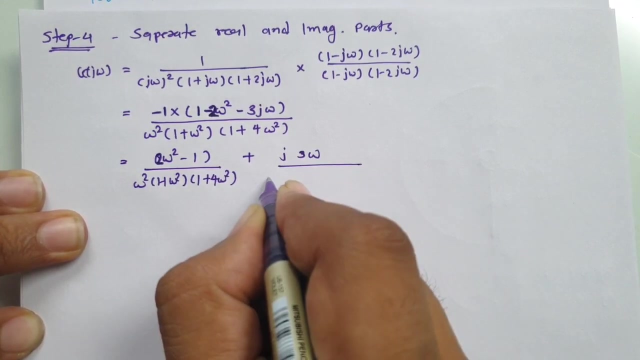 Right, So 1 plus the Real, So 1 square j. when you write it will be represented in R as the 2 square j. when you write it into 1 square t, square 0, we will need to add it, so to show it again in R such a: that is what. 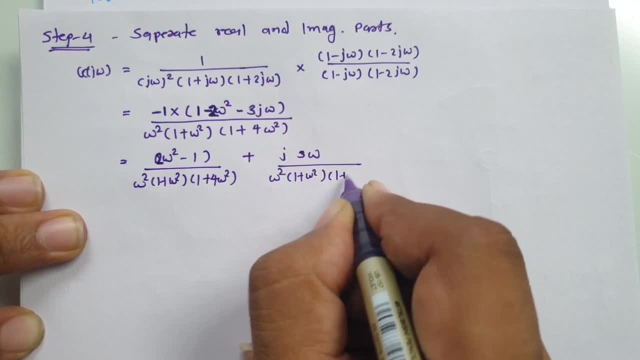 we will need to compare anyway. Okay, So now we have this w squared, This one. you have to solve this problem. So this all right, then now you go to the second equation. Okay, You are going to take this to the help ruling. 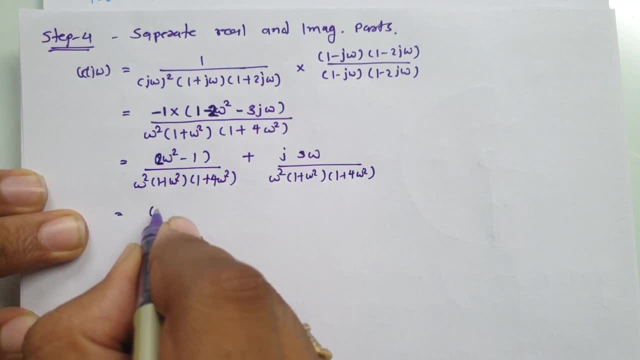 And you have to interact with fl. Okay, At any point of time, you won't have to take further the look. It's most important one is that you find out when you do what you've said. now let us further simplify this. so 2 omega square minus 1 divided by omega square into 1 plus omega. 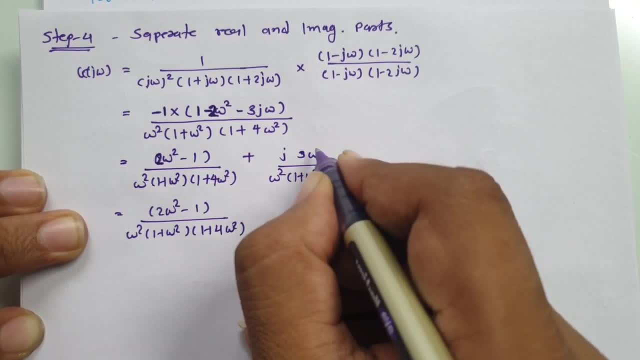 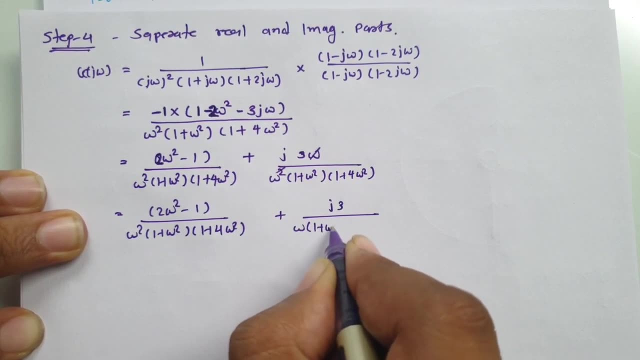 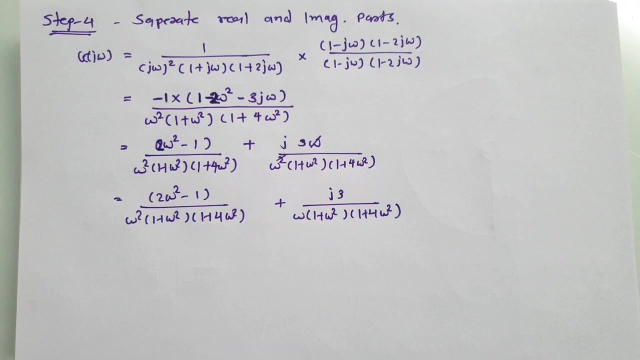 square into 1 plus 4 omega square and this omega will get cancelled. so plus j3 divided by omega into 1 plus omega square into 1 plus 4 omega square. right now to identify intersection to real axis, imaginary component that is 0, and to identify intersection to 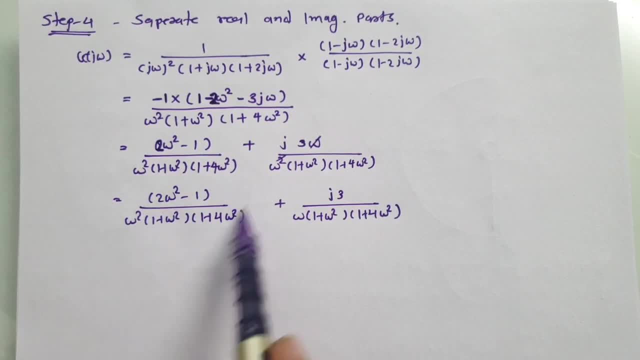 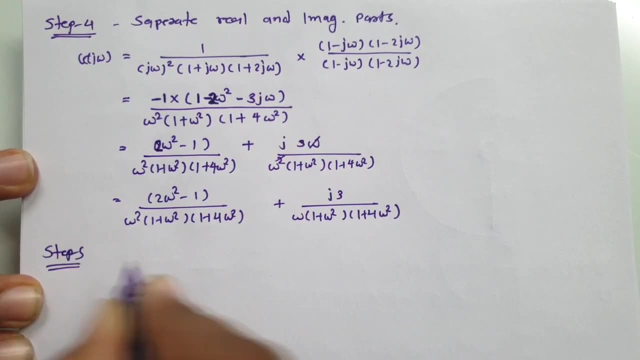 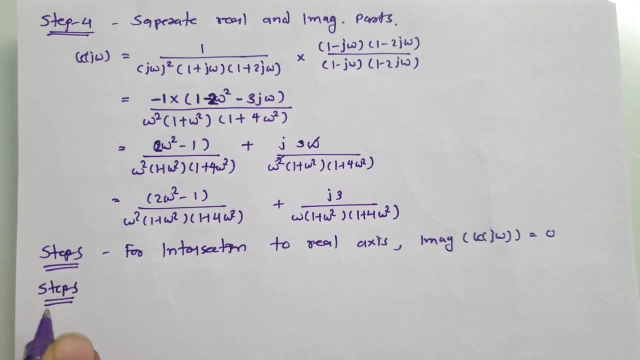 imaginary axis. real component of this should be 0, right? so let us identify intersection to real axis. and if you have this, there is no intersection, you can see, right. so we can say: let us try it for intersection to imaginary axis. So for that, this part, that should be 0.. So 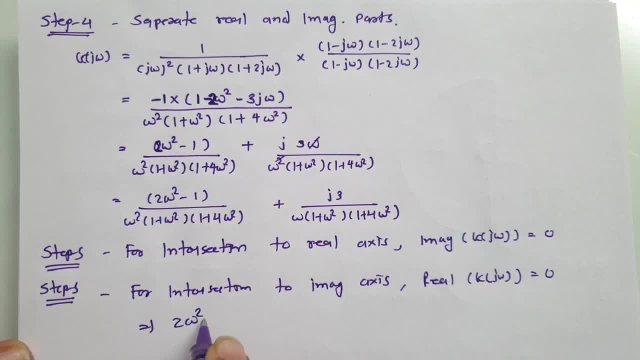 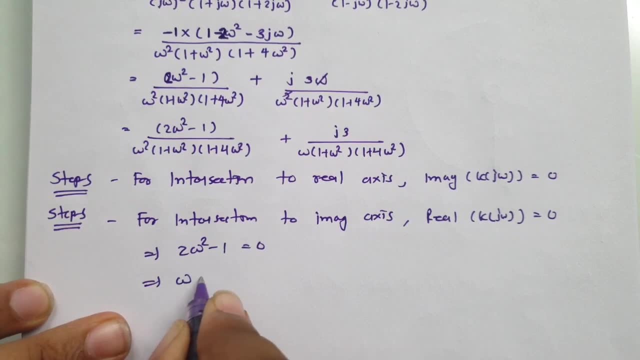 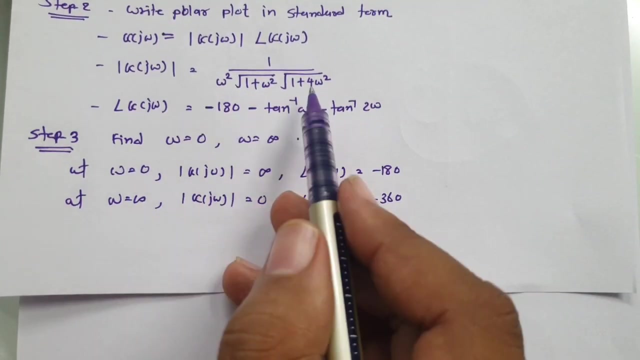 if you equate this is equals to 0. we can say: 2 omega square minus 1. that is equals to 0, and that will result into: omega is equals to 1 by root 2. that will result into: omega is equals to 1 by root 2.. Now see, if you place omega is equals to 1 by root 2 in magnitude. 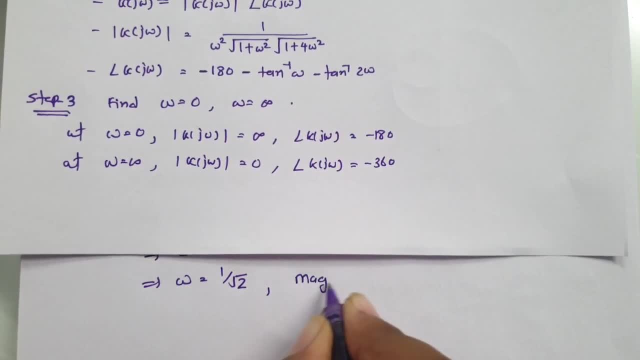 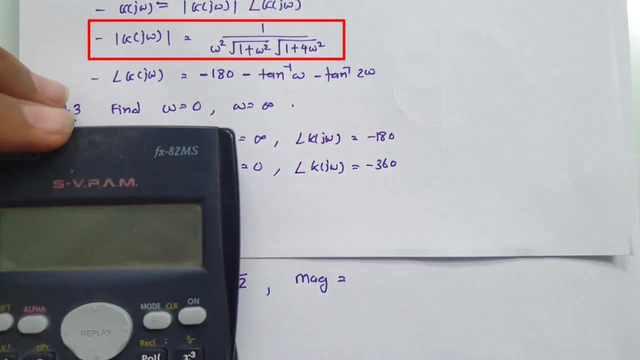 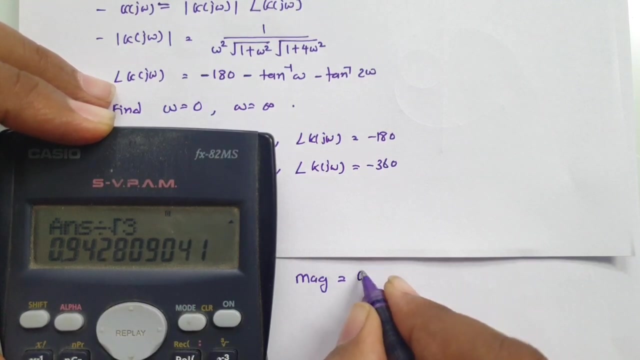 then we'll be having a magnitude right, So magnitude will be. now. you see I am placing omega is equals to 1 by root 2 in this right, So magnitude is 0.94, right. And omega is equals to 1 by root 2 in this, So omega is equals to 1 by root 2 in this. 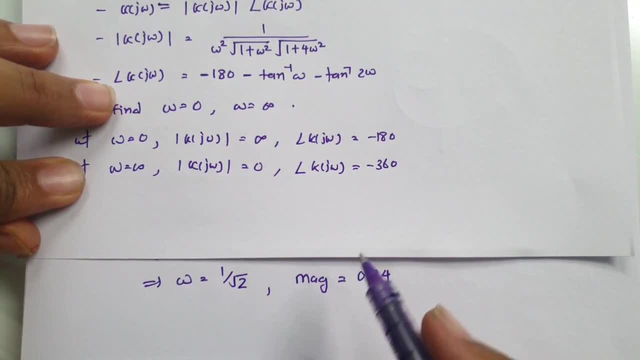 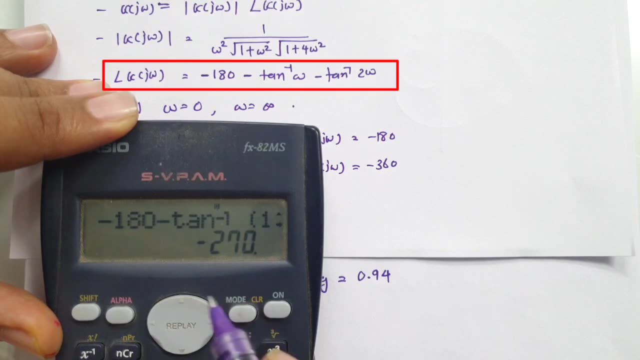 And to have phase at this frequency we need to place omega 0 to 1 by root 2 in this. So let us place it So this is having angle minus 270. So phase is minus 270.. So now we got the intersection to imaginary axis right. 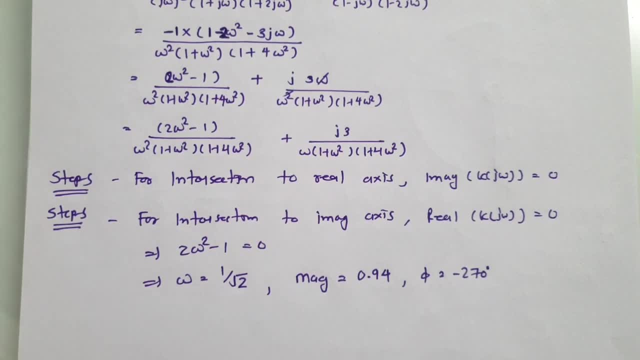 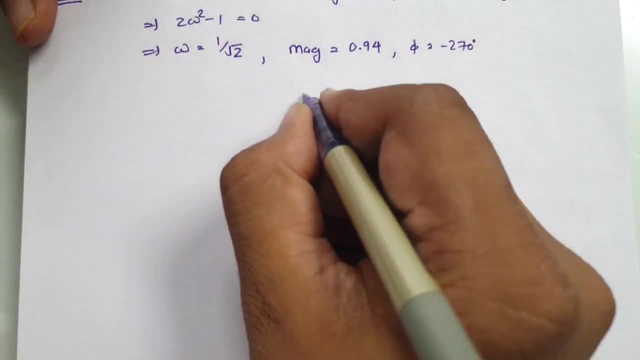 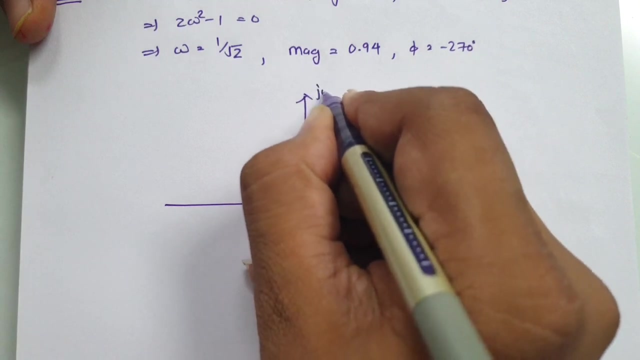 Now we are delivered to plot Nyquist plot, step by step, right, Right. So in Nyquist plot, as I have told you, first of all we need to have polar plot right. So let us have that over here. 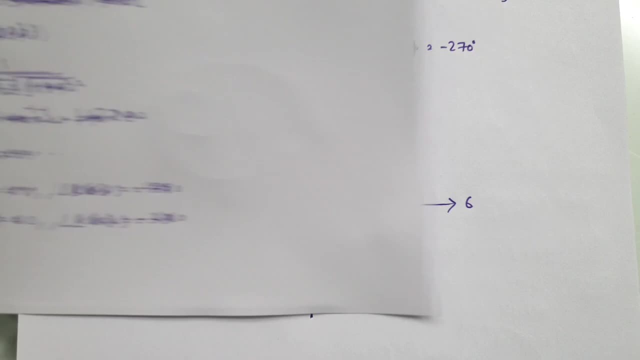 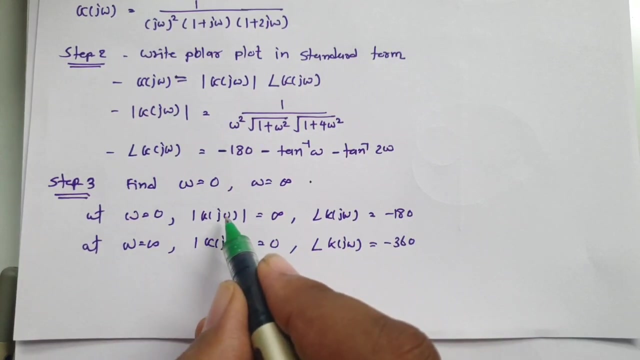 And you see, for polar plot, two essential points that we have identified at: omega is equals to 0. Phase is minus 180 and g of j omega. So magnitude is infinite right? So here minus 180 is happening, right. 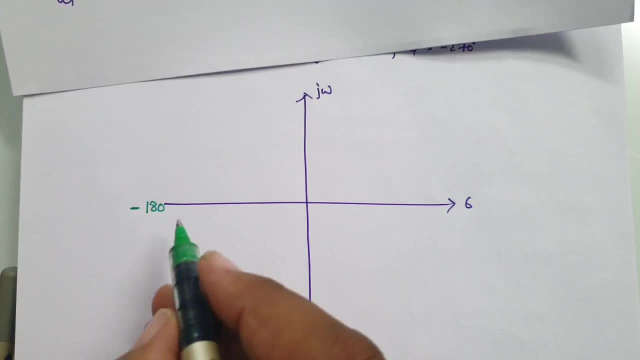 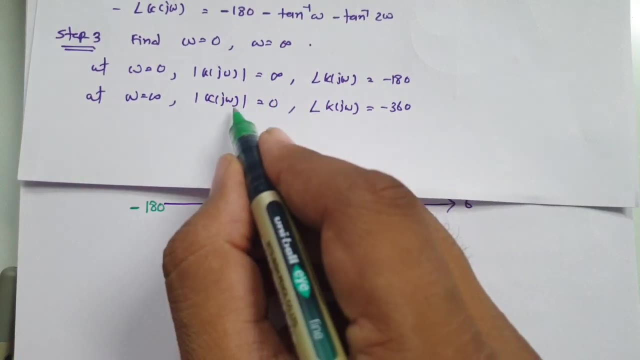 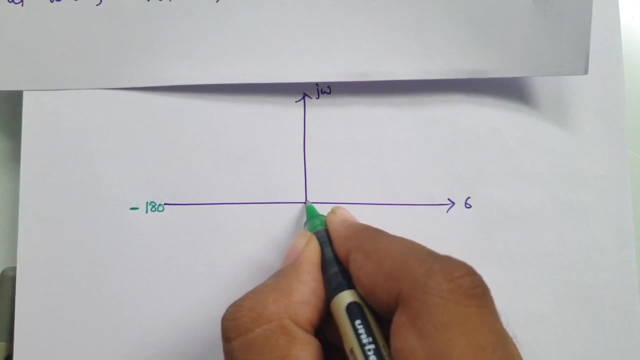 So here minus 180 is happening and magnitude is infinite, right, And at omega is equals to infinite. we have magnitude 0 and angle 360, right. So from 360, it is coming over here, From 360, it is coming over here, right. 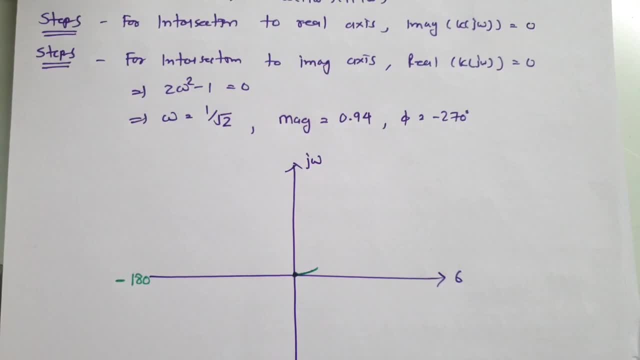 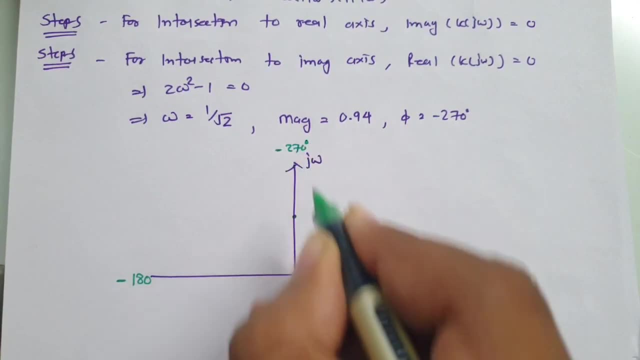 And if you see intersection to imaginary axis, that is happening somewhere over here at minus 270 angle. So here minus 270 angle is there and this is having magnitude 0.4.. So distance from center: that is 0.94, right. 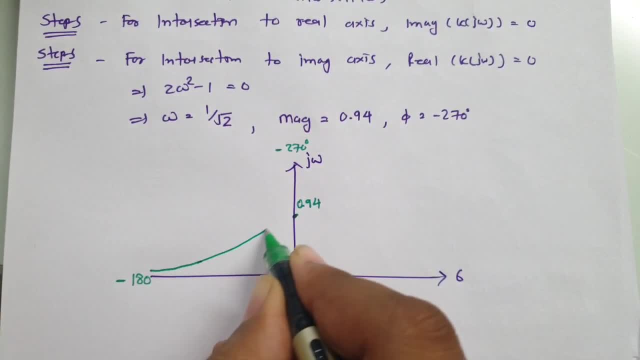 So you see, it is happening like this. It is happening like this, right? So this is my polar plot, Where here omega is equals to 0- that we have. and here omega that is equals to infinite- that we have right. 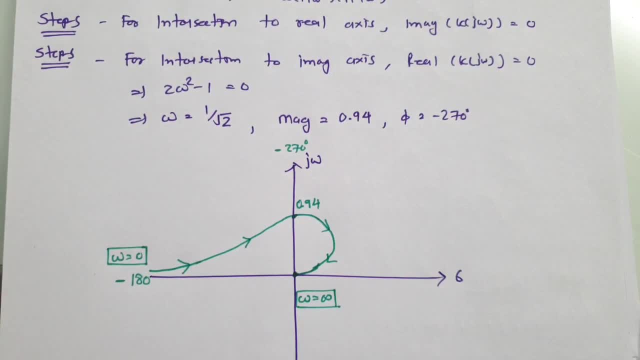 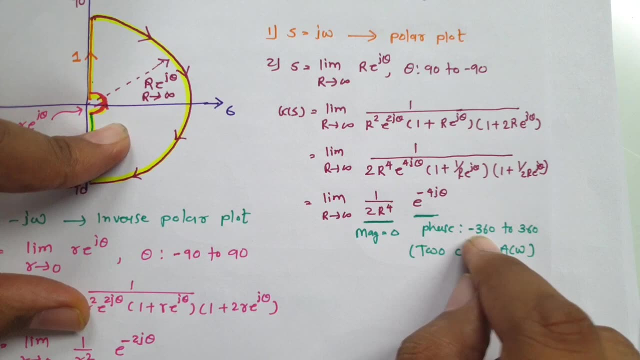 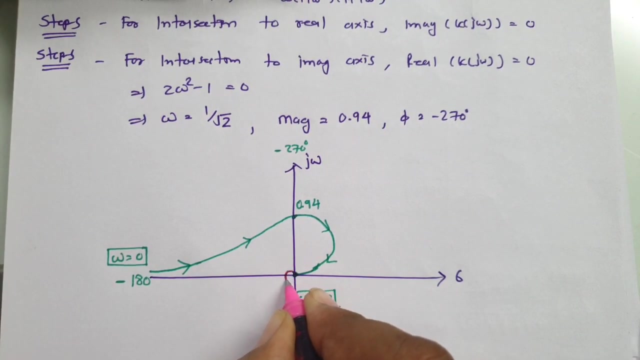 Now, next step that we have calculated, that is there, with magnitude 0 and phase minus 360 to plus 360. What it means: Two circle in anticlockwise direction. So this is one circle and this is second circle and it should be having 0 radius. but to show you, I am just making it this big right. 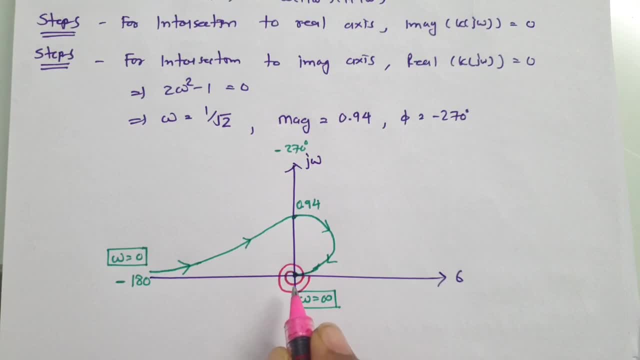 Else it will be very small circles, which is having radius almost 0, right. So that is there in anticlockwise direction. remember It is there in anticlockwise direction. So this is our second portion. Now if you observe third portion, so that is to plot inverse polar plot, right? 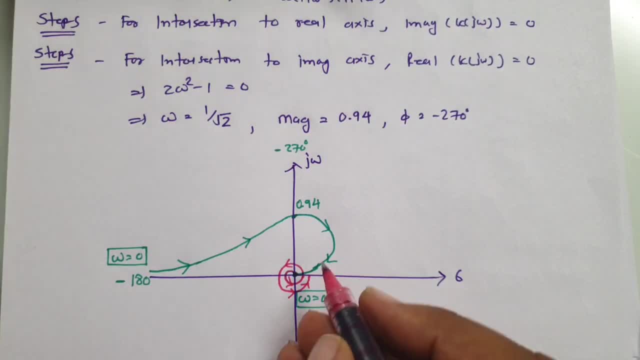 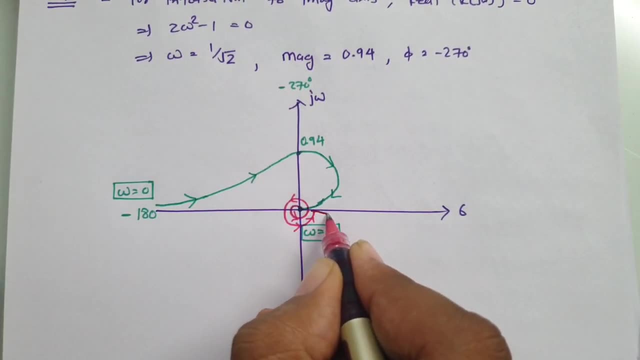 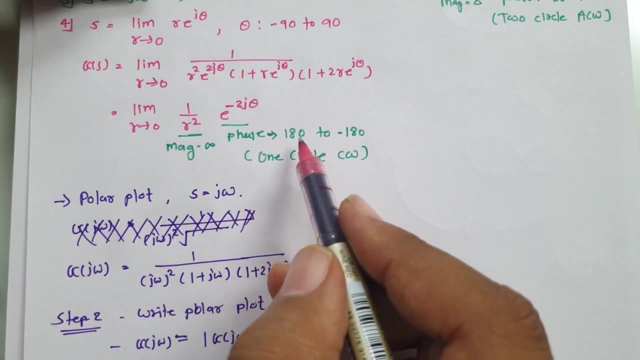 So let me plot inverse polar plot here. So inverse polar plot, so that is inverse of this. So inverse of this will be like this, you see. So this is inverse polar plot. and in fourth step I have explained: magnitude is infinite and phase is varying from 180 to minus 180, so that is there, in clockwise direction. 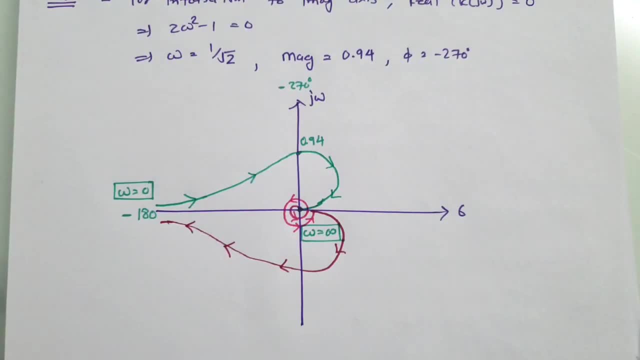 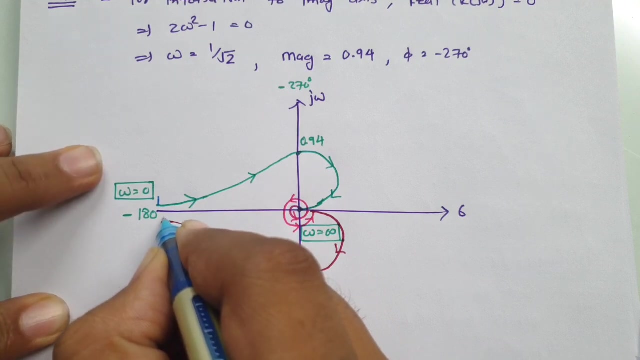 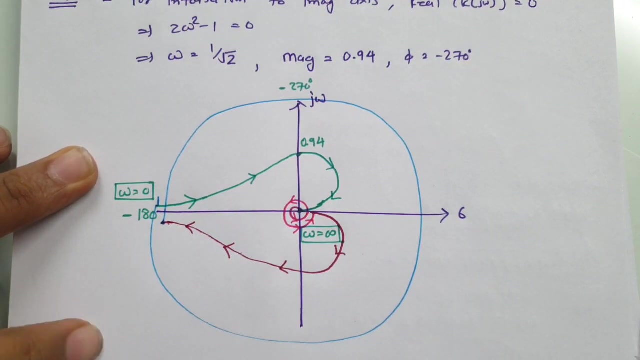 So phase will vary from 180 to minus 180, so you see, this is 180 and it should be there in clockwise direction. So you see, from here it should go like this, with infinite radius, and it should get connected over here, right? 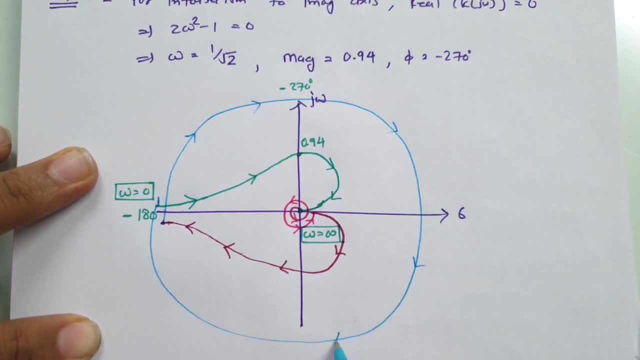 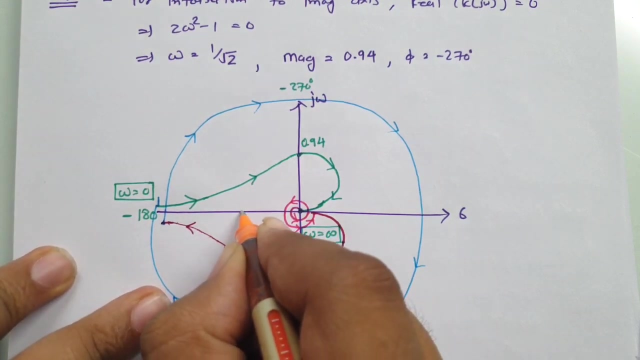 So you see, it is there in clockwise direction. So that is how complete Nyquist plot is there with us right Now. there is one more question, That is to identify, Identify, stability. So you see, here we have a critical point. 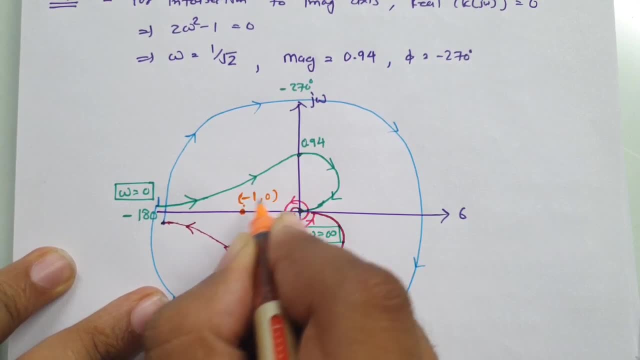 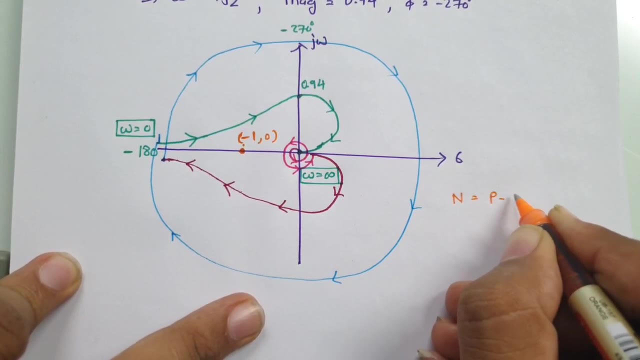 Let us say this is minus 1 comma 0. That will identify stability. Now for stability, we should know: n is equals to p minus z, where n is n-circlement, p is number of poles on right half plane for open loop system. 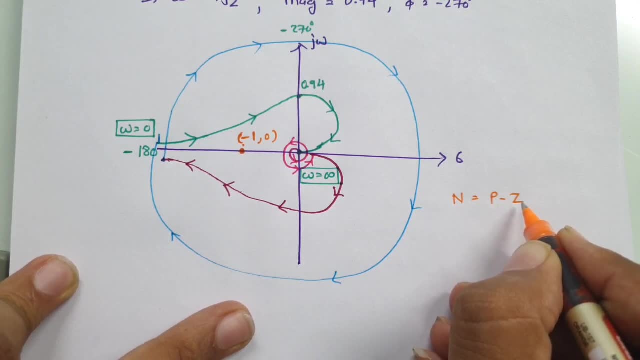 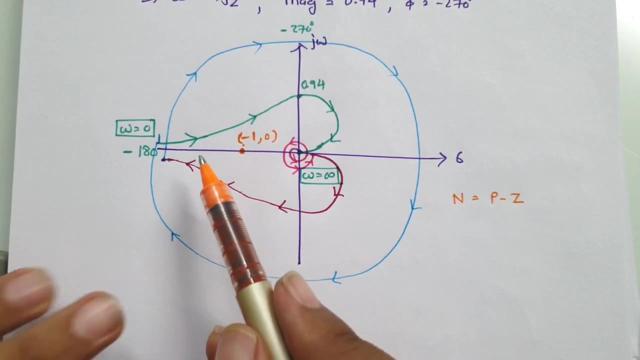 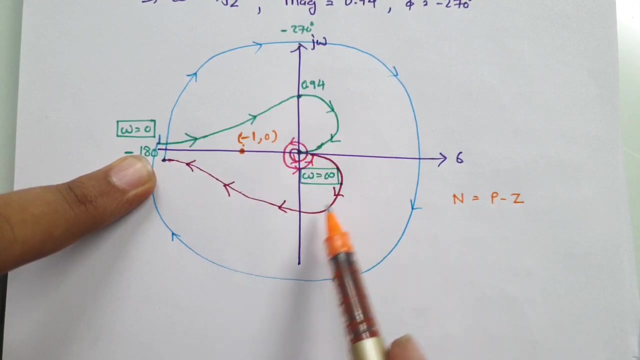 And z is number of poles on right half plane For closed loop system. So let us identify n? n-circlements. So you see, here, if you observe, this is one n-circlement that is happening. You see, that is one n-circlement and that is happening in clockwise direction.